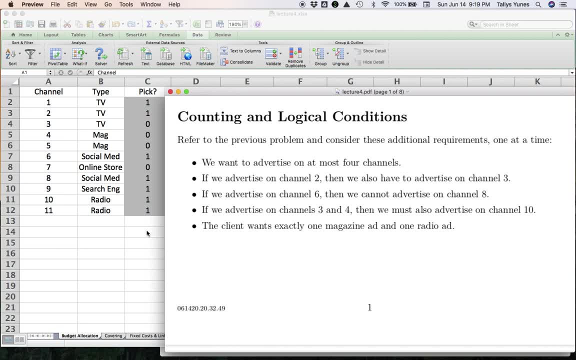 the client says no, that's too much or too many. i would like to restrict the advertisement to four different channels at the most, so that it's not too many over. so they may have a reason to request something like this. another typical example of this type of constraint is, let's say, 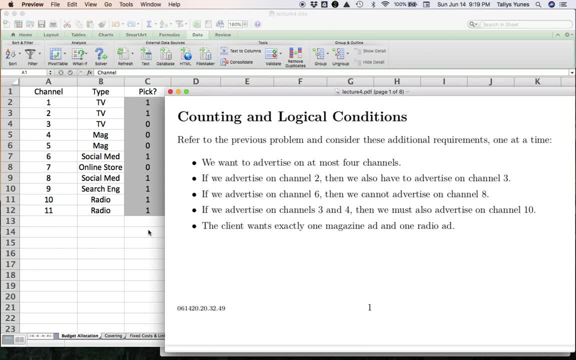 you're building a portfolio of stocks and if you just solve the plain optimization problem, you get a solution that you know invests into 200 stocks and many of which could be very little money in them. so maybe you want to impose, you know what? give me the best portfolio that uses only let's. 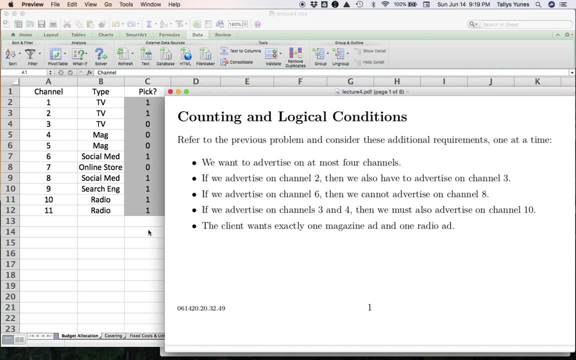 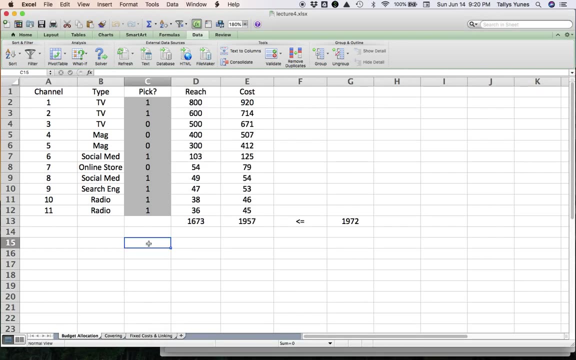 say, 30 stocks. so you want to count how many, you want to count how many, you want to count how many times you were doing something and limit that number. this is one situation where you need the binary variables and we have them here already and we simply have to count. well, when you add, 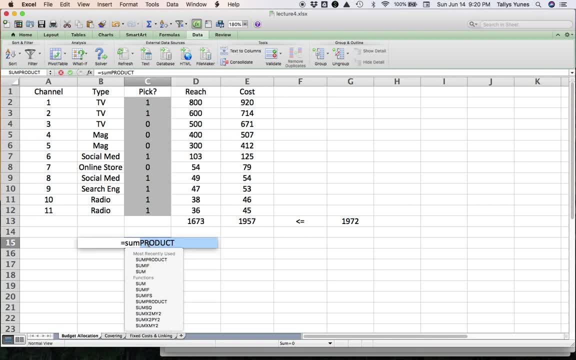 binary variables together, interestingly because they are zero ones. what you get as a result is always going to be how many yeses there were. so if you add binary variables together and you limit that sum to a number, you are essentially limiting how many yeses can there be, and in this, 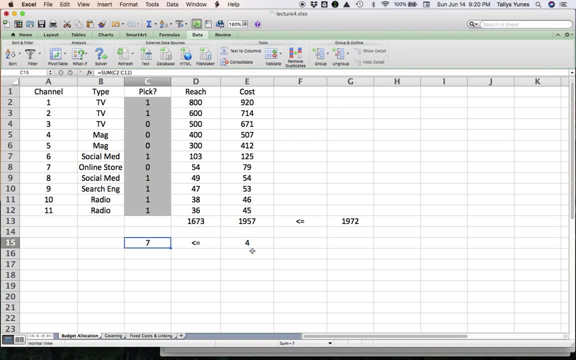 case the client said i wanted the most four yeses out of these potential 11. yes, no variables right now. as we counted we have seven. that's why there's seven here. so in that cell i simply summed them so i could go to solver and add one more constraint by simply saying: you know the sum of the. 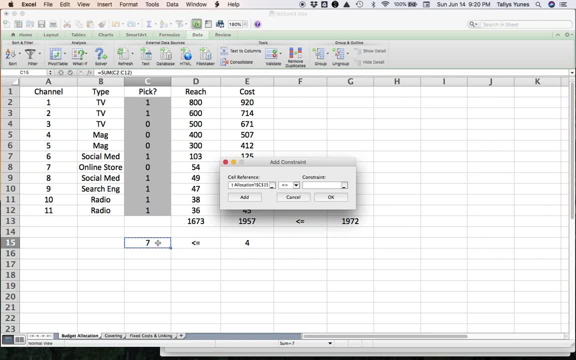 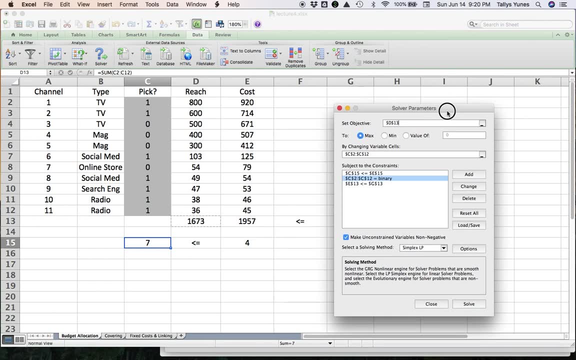 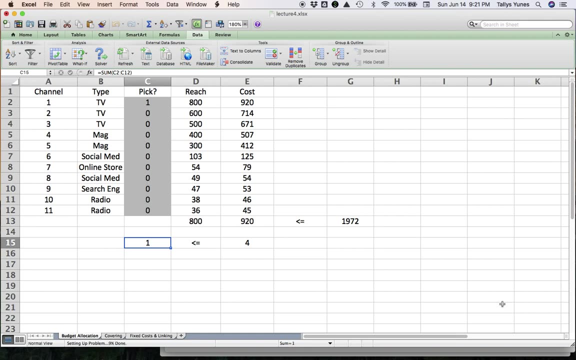 binaries is, at the most, what i want to allow for. okay, and if i solve this, what i'm gonna get as a result is the collection of the four best ads that stay within my budget and reach as many people as possible. okay, so, and here they are. all right, it's just a very simple way to get to the bottom of the. 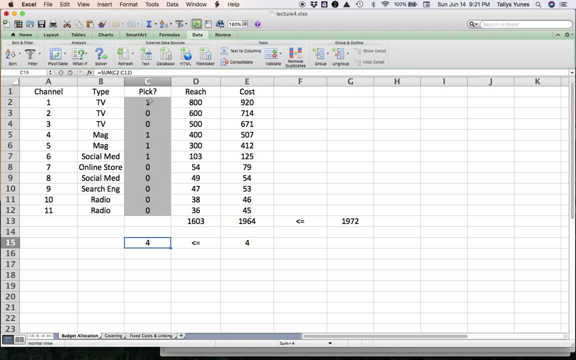 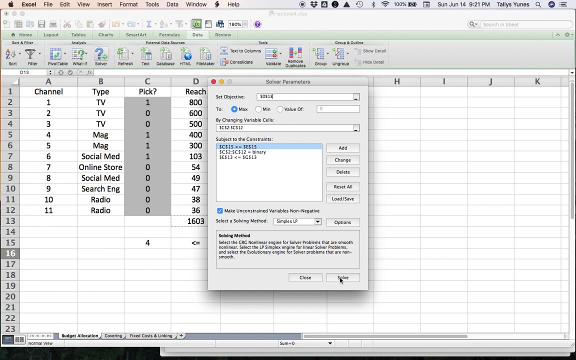 list. so here we have the first two magazines, the first social media ad and the first tv, and that's the best you can do if you're restricting yourself to four. okay, so let me go back to the other, the initial solution, because the following logical constraint examples i want to show you will be: 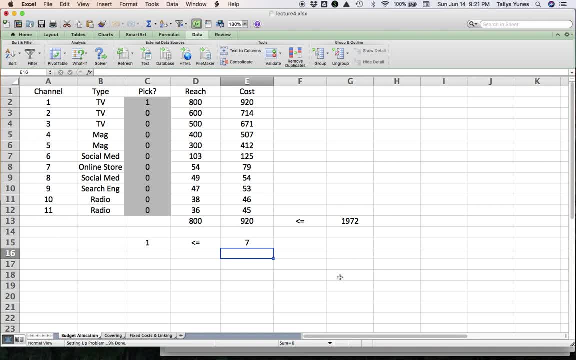 more, more meaningful, if we have the, the bigger solution at hand. so here we are. we were already here in the initial solution and the first solution was quite simple. in this case, we we were able to use the best four ads. now we need to go back to the networks that we've been looking. 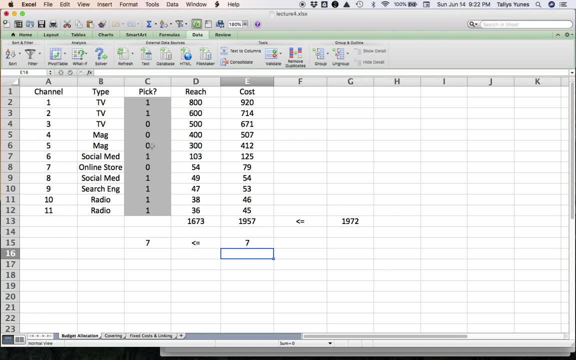 at. let's say this was our previous solution and notice, the solution with the best four ads is not a subset of the solution with the best seven ads. and this may be a little counterintuitive for some because, notice, the solution with four ads was using these two magazines, wasn't it? 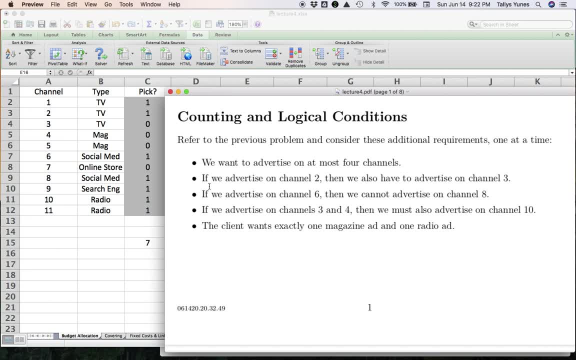 here's a condition of the type: if this, then that, and it says the following: if we advertise on channel 2, then we also have to advertise on channel 3. ok, right now, you see, this is not happening. I'm doing channel 2, but not channel 3. 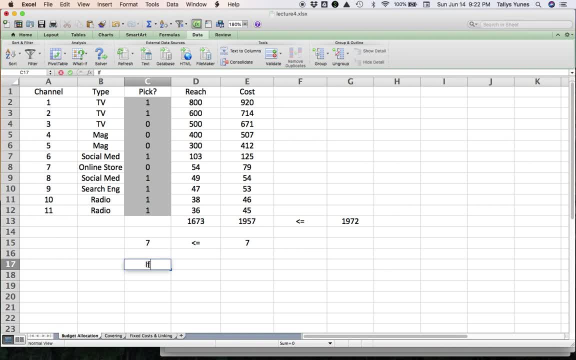 if this, then that condition. if channel 2, then channel 3. right, if x2 is 1, then x3 has to be 1. if this is a yes, then the second one has to be a yes. if this is what you want, there is a way to write this down as a formula. 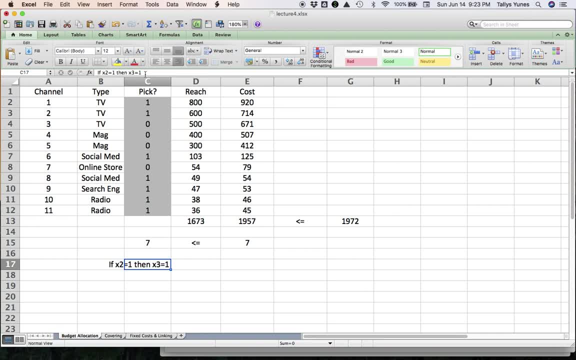 we're going to deduce this in class, but for now I'm just going to use the one directly, because we don't have too much time. if we have a condition like this- and the x's are, and I don't know why this is coming up- 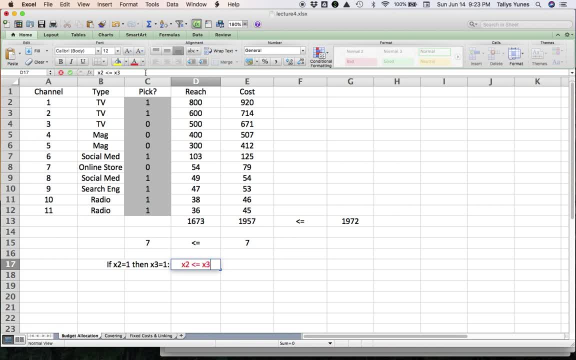 red, but that's ok. if the x's are binary variables, the formula for it is always going to be this one. if you want to do, if this certain thing is a yes, then this other thing is also a yes. the formula will always be the binary of the first thing. 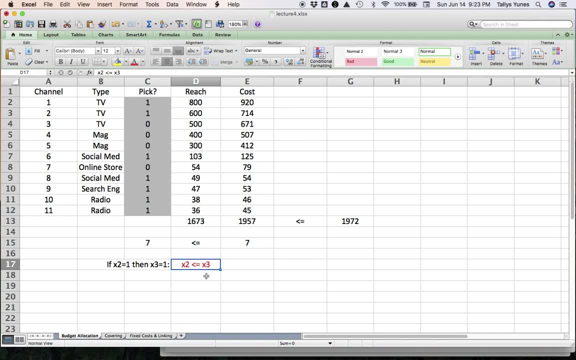 less than or equal to the binary of the second thing, because this essentially disallows the first one from being a 1 and the second one from being a 0, because 1 is not a 0 less than 0, no matter what the story is. 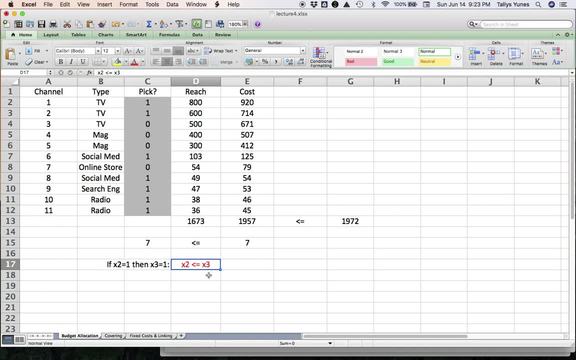 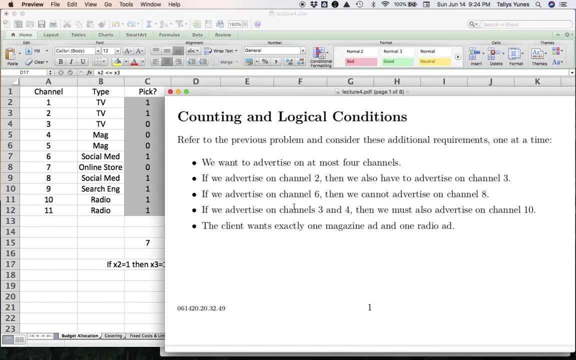 what the situation is if you have two binaries and you want if this, then that it is always going to be this formula: the x of the first thing less than or equal to the x of the second thing. our next one is a mutually exclusive example and it says: 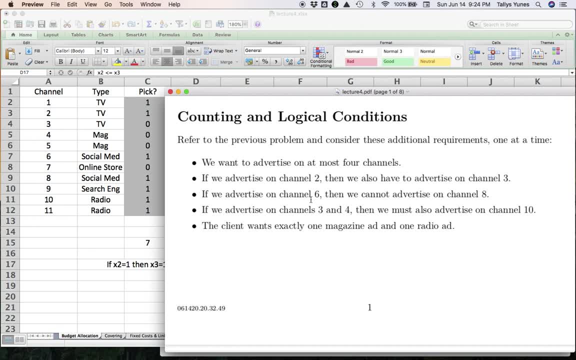 if you advertise on channel 6, then you can't advertise on channel 8, and you see we're violating that as well. here we're advertising on both 6 and 8. so if what you want to write is the following, and let me copy this: 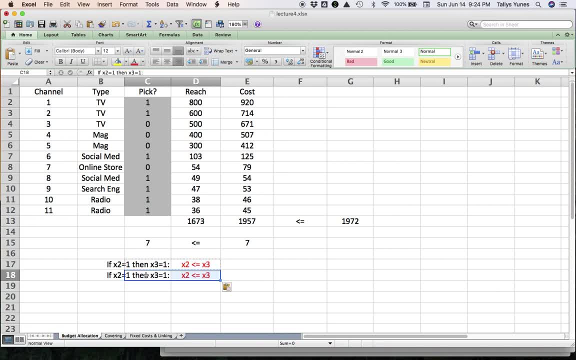 just save some time. the second thing I want is: if you do 6, then you can't do 8. this is what the story says there. so essentially, what you want is if 6 is a yes, then 8 has to be a 0. the formula for it is: 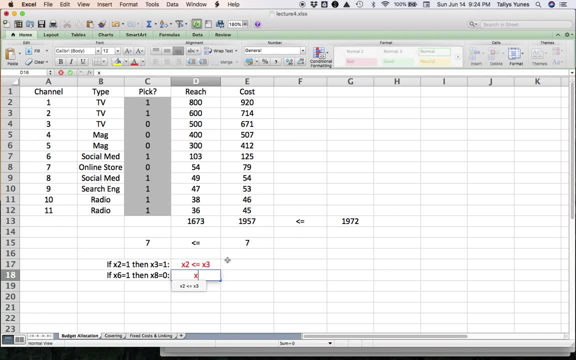 and it's generic, like the previous one. no matter what the situation, if you have two yes-no decisions and you want them to be mutually exclusive- that is, if one happens or if one is a yes, the other one has to be a no- your formula will always be this: 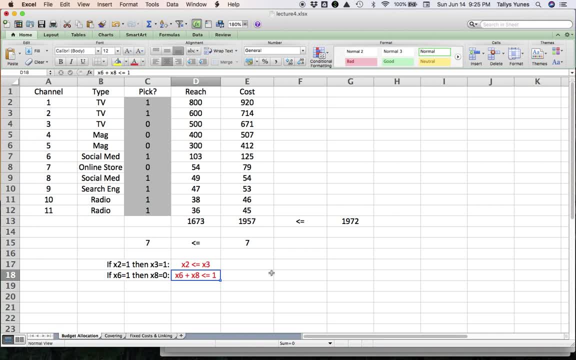 the sum of the two binaries at most 1, because what you want to eliminate is the yes-yes answer, the 1-1. so 1 plus 1 would be 2, which is not okay for this formula. so this formula is excluding the yes-yes answer. 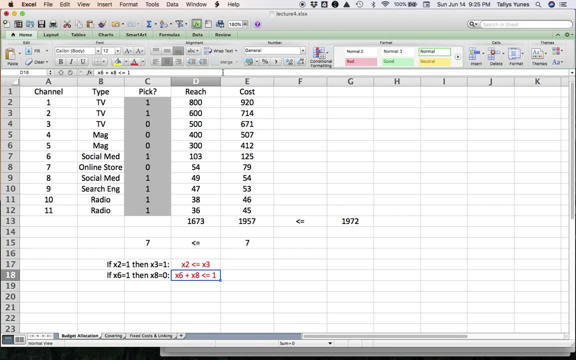 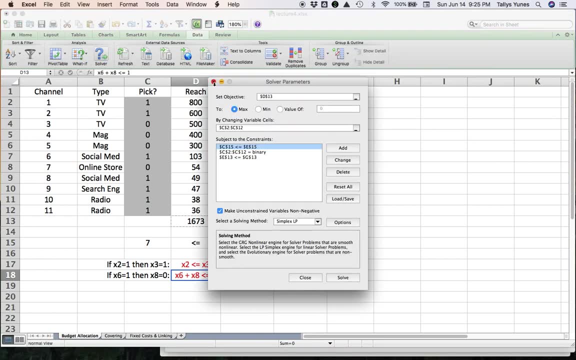 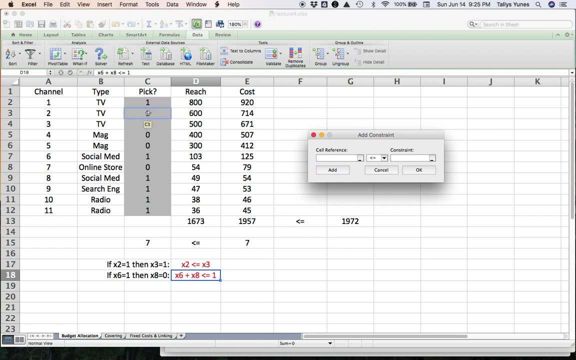 well, if you wanted to put these into solver, you simply implement them as they are written here. so let me just show you, for example. if we wanted to enforce these in this particular example, we would do this. we would want x2. x2 is c3, less than or equal to. 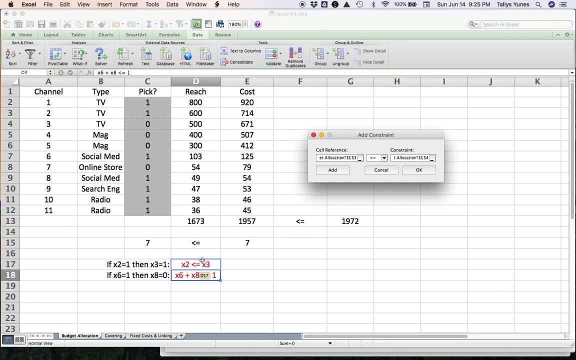 and x3 is c4. that would implement the yes-yes answer and the if this, then that condition. and the other one is we want to say: well, in fact, in this case, because there is a formula here, we need to first produce this formula in excel. 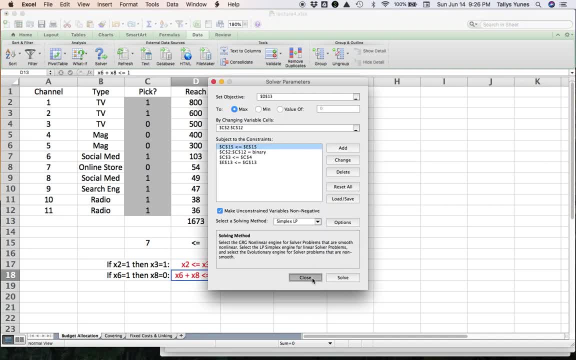 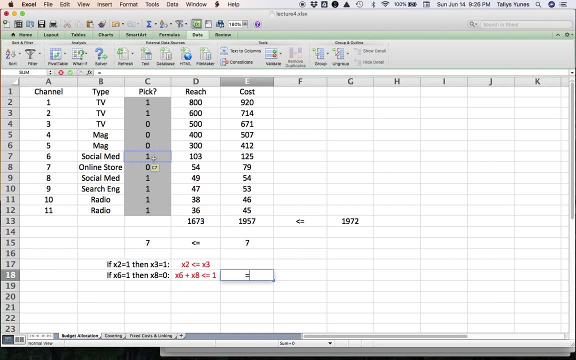 let me get out of here and go ahead and do it. so here I'm going to create the x6 plus x8 expression: x6 is c7, x8 is c9. right, and this is what I want. to make less than or equal to 1. 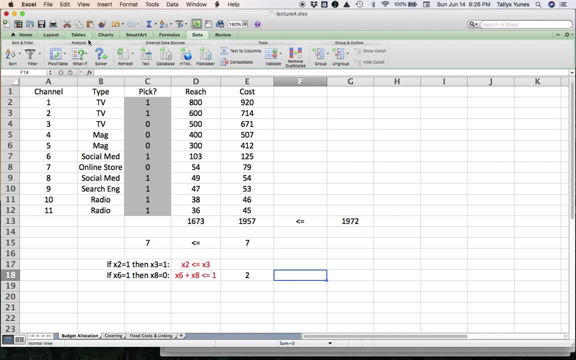 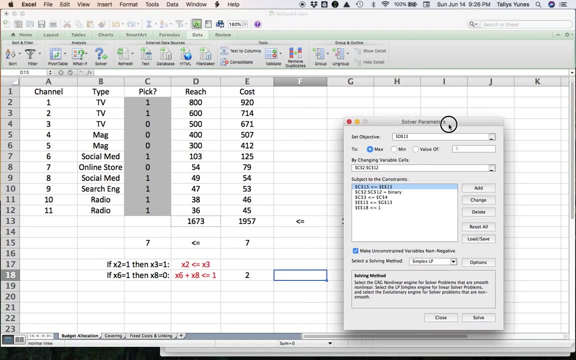 right now it's a 2, so it's violating the requirement. if you go into solver, I could go ahead and say one more constraint that says, hey, this number has to be at the most 1, right? so I have imposed these two additional conditions in red. 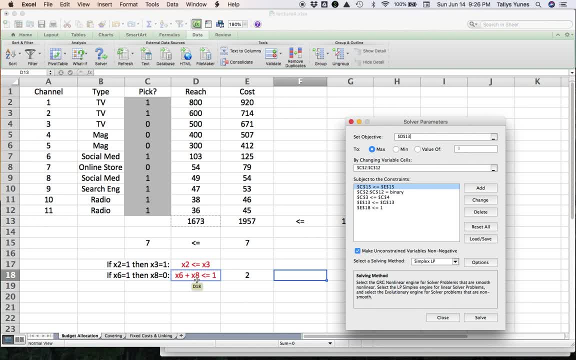 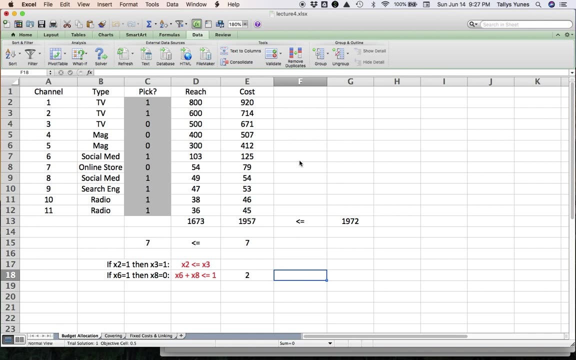 or constraints which are currently violated by this solution. so the new solution will, of course, be different. let's see what happens. I have no idea if this is going to work, because it might generate some contradiction, but I don't think so. we'll see. yeah, so here we go. 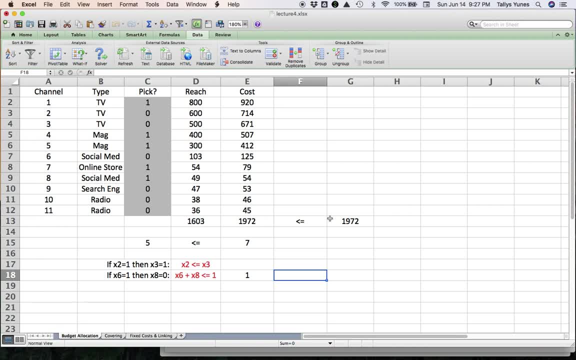 let's see if it respected what we wanted. budget is respected. okay, good, we have the following: x2 is a 0, so I chose to do neither. if you have to do this, you have to do. if 2, then 3, the answer is neither, and if you do, 6. 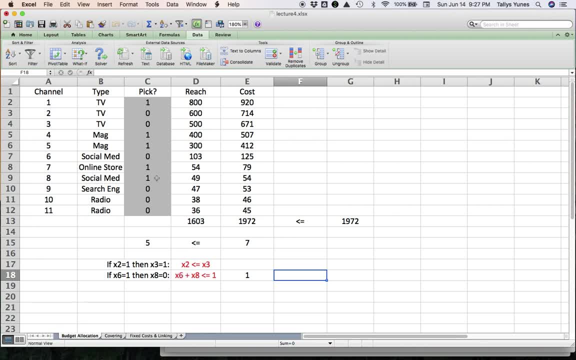 you can't do 8, and here we are not doing 6 but are doing 8, which again is obeying this requirement. so we are good here and our maximum reach is 1,603,000 people, and we have matched the budget and we are now advertising. 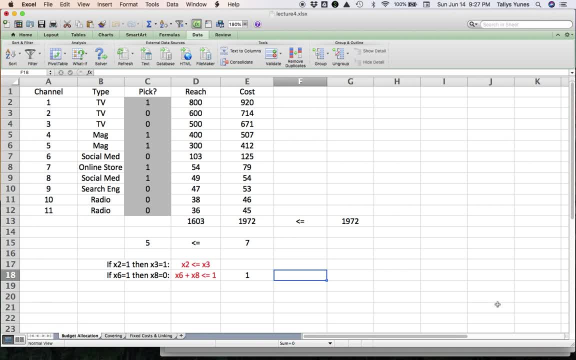 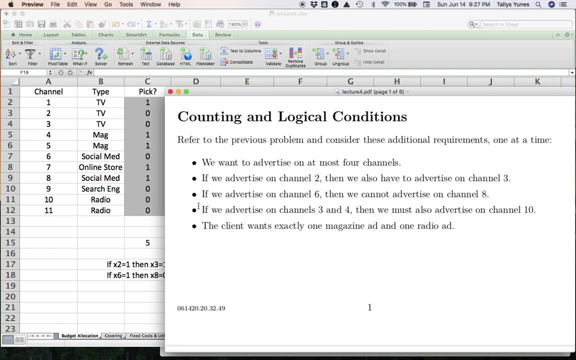 on 5 channels instead of 7. great, let's see. I think there's a few more here. this fourth bullet is the third most common type of logical condition that you might encounter in a real life problem from my personal experience. so these first two are very common. 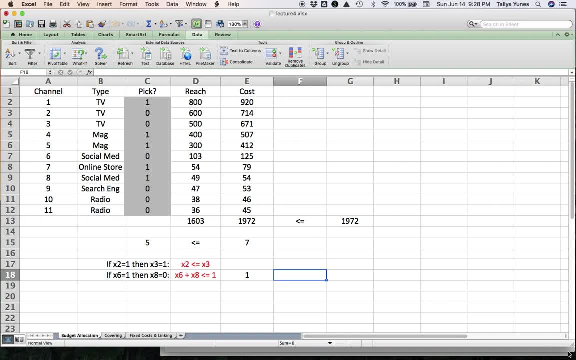 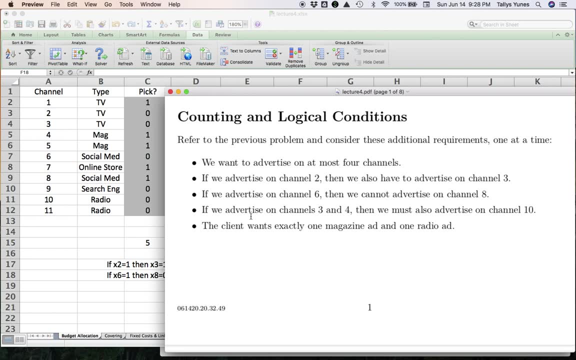 if this, then that, if this, then not that. the third one that I would say is the third most common is this one that involves three variables. and this one says: if you advertise on channels 3 and 4, okay, if you do these two things, then you must also do. 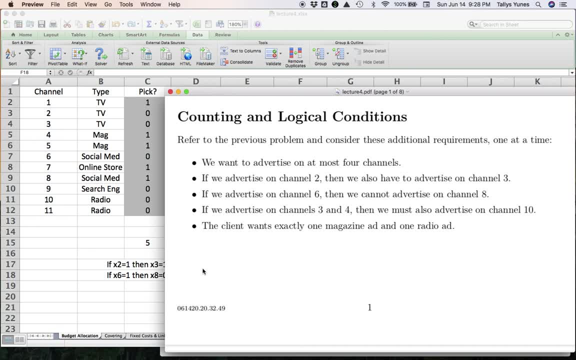 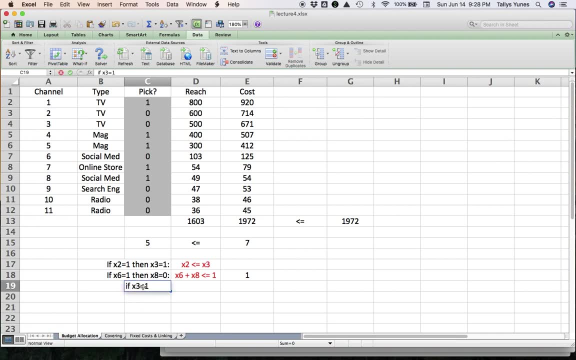 a third thing, which is advertise on channel 10. so this is, if this and that, right. so if you advertise on 3 and you advertise on 4, then you have to advertise on channel 10 and this one again. we could do some calculations and try to deduce. 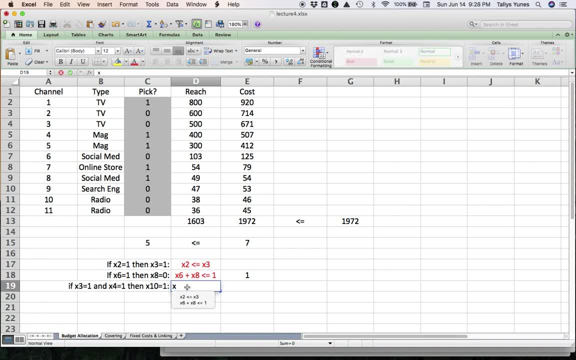 what the formula will be, but I'm just going to give it to you, as I did with the other ones, and the idea is the following: what you want to avoid or enforce is that if both 3 and 4 are equal to 1- and let me make this red- 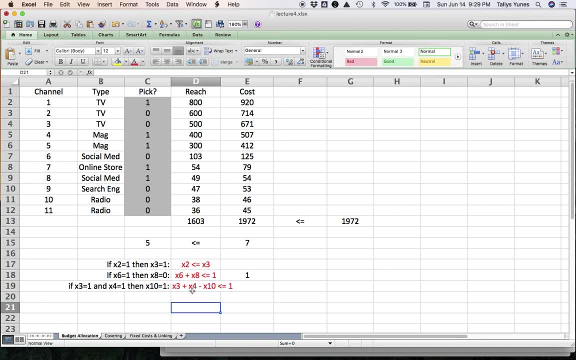 so that it's consistent with everything else. if both 3 and 4 are equal to 1, x10 doesn't have a choice. it must be 1 as well, right, if you did yes, yes, you want to force x10 to be a yes, and the way 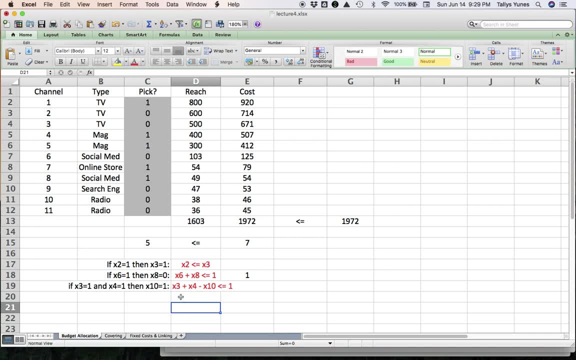 this formula makes that happen is this: notice that if this is a 1- 1, I have a 2, but I have a less than or equal to 1, so this guy here doesn't have a choice because I need to do 2 minus 1. 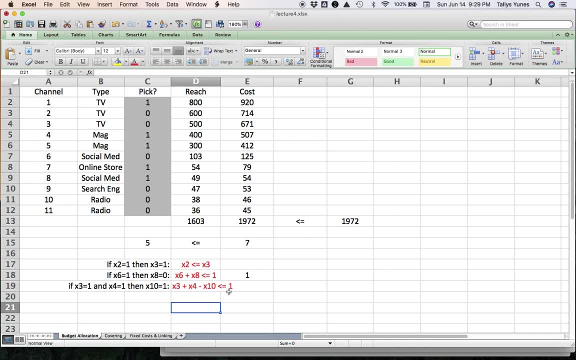 to satisfy the less than or equal to 1. so when you put 1 and 1 here, x10 is forced to be 1 and in any other situation, no matter what you put in, 3 and 4, 0, 0, 0, 1, 1, 0. 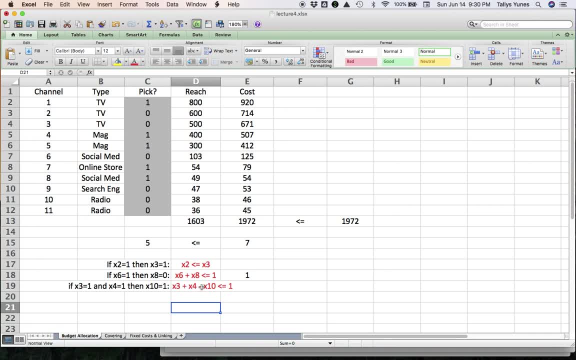 you're not going to need to force x10 to be anything. x10 is free to be any value. okay, so if you ever face this third situation again, no matter what the story is or context, financial context, marketing context, doesn't matter, you have 3 and 4. 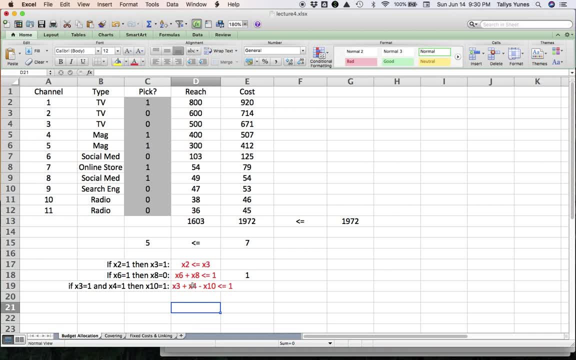 x10 is free to be any value. you have 3 binary variables. if 2 of them are yes, a third one has to be yes. this will always be the formula to use, so you can add that to your utility belt that you carry around with you to model optimization. 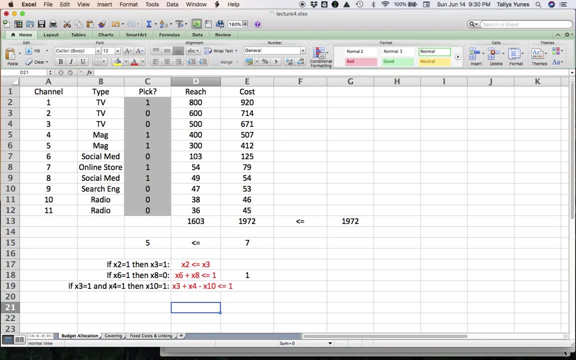 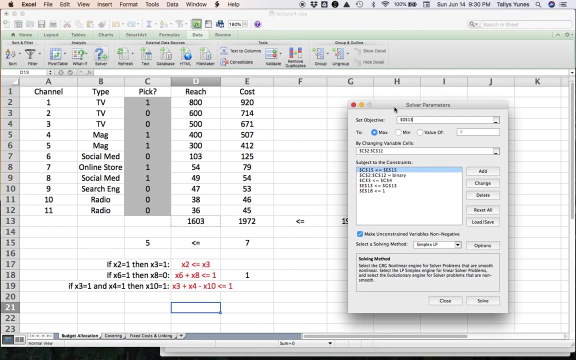 problems in real life. excellent, let me see. I think there is one final example I wanted to do with you, and again, let me go back to the original solution, because this will make more sense if you go back there, and then that will be the end of this video. so I'm going to remove. 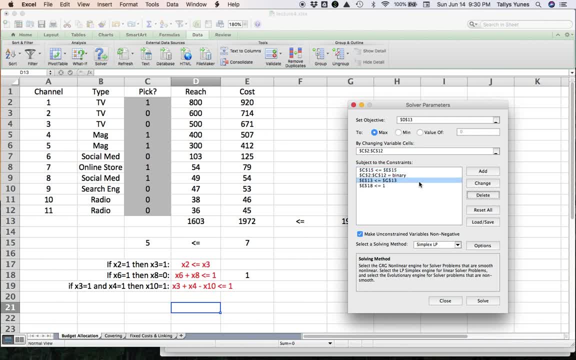 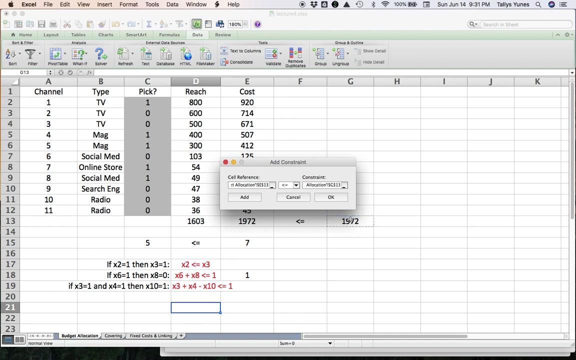 this one and I'm going to remove this one. yeah, and we just stay with the original. I think I removed the wrong thing, right? yes, probably so. let me just add it back. I just need to add the budget constraint back. I already had the binary constraint. if you solve this. 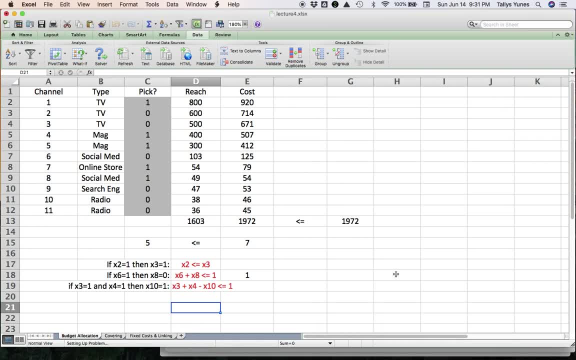 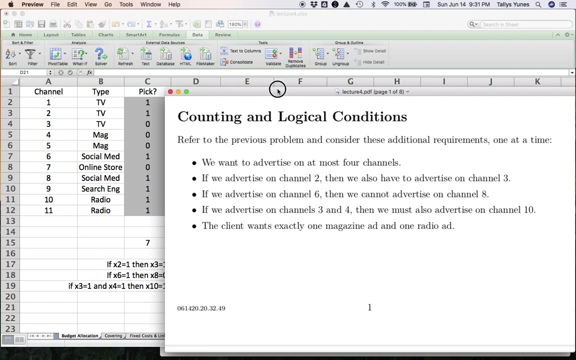 let's just make sure we go back to the first answer: yes, ok, so here we are, and the last example of one of these conditions that I want to do with you is the following: the client looks at this answer and goes: you know what I really wanted. 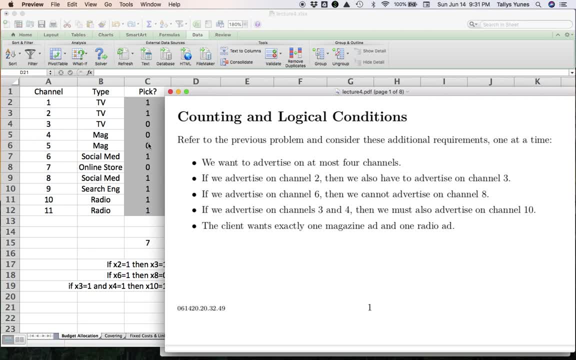 to have an ad on a magazine and you're coming back with no magazine ad, and I think two radio ads is too many of the same type, so I want to add more diversity to this. could you find me an answer that picks one of the two radios? 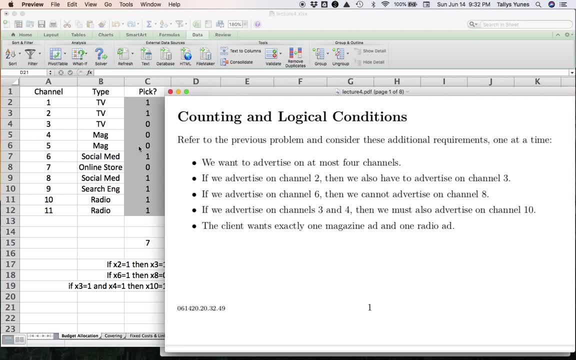 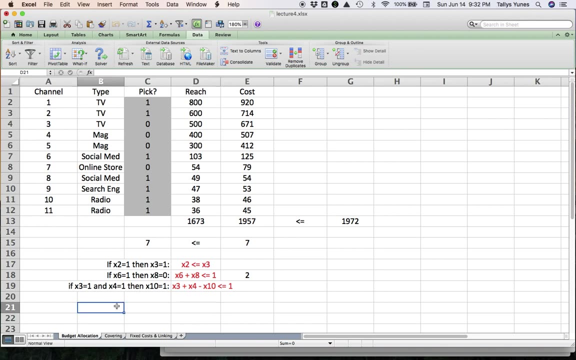 I don't care which- and also picks one of the two magazines- I don't care which and give me the best answer that satisfies those two requirements. right? client wants exactly one magazine and one radio ad. great. so what you could do here is the following: you could say: 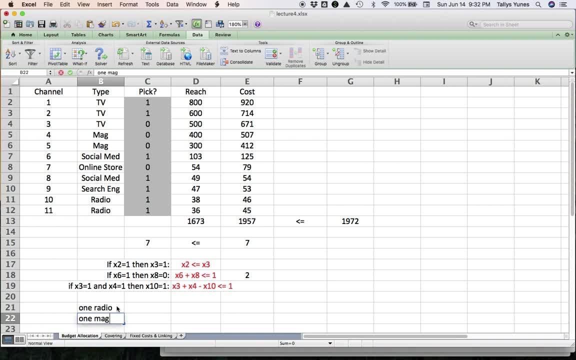 they call this one radio, one mag. so essentially what you want is you want these two variables here to be one of them a one and the other one zero, so you want the sum of them to be equal to one. you don't want the sum to be two, because that would be two yeses. 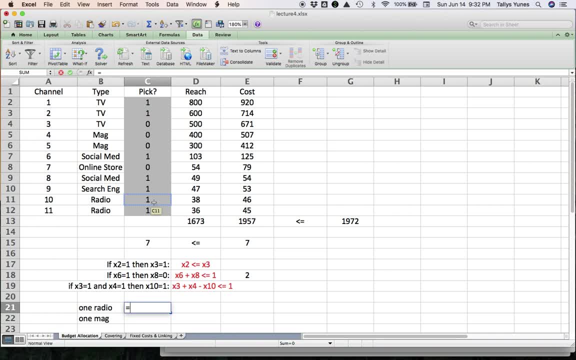 and you don't want the sum to be zero, because that would be two no's. so what you would like is: you would like this variable plus this variable right to equal one and same thing for the two magazines. you want this variable plus this variable to equal one. 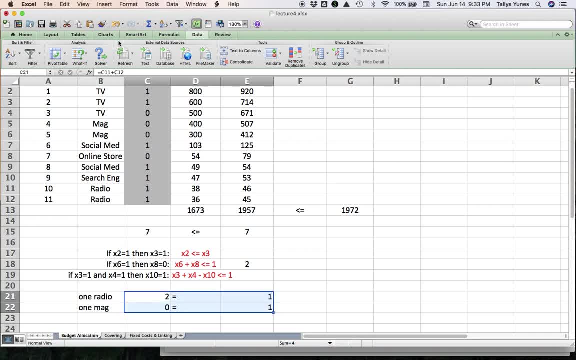 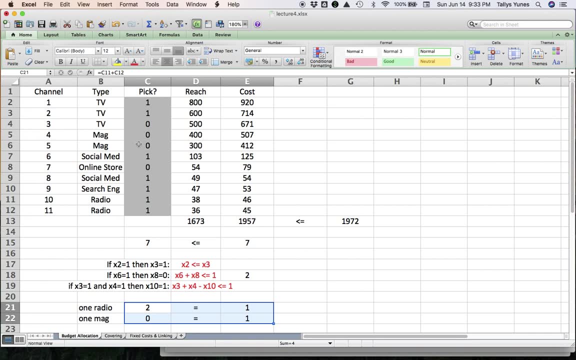 right. so the constraints you have imposed, mathematically speaking, are x4 plus x5 equals one and x10 plus x11 equals one. and notice that the current solution violates this one because now you have two yeses and you want one yes. and it violates this one because 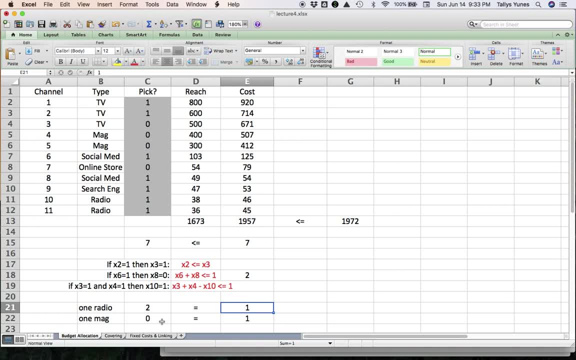 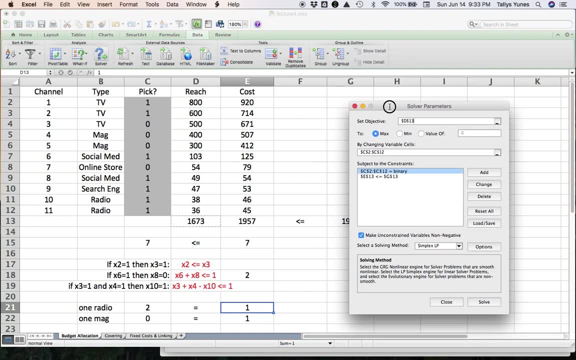 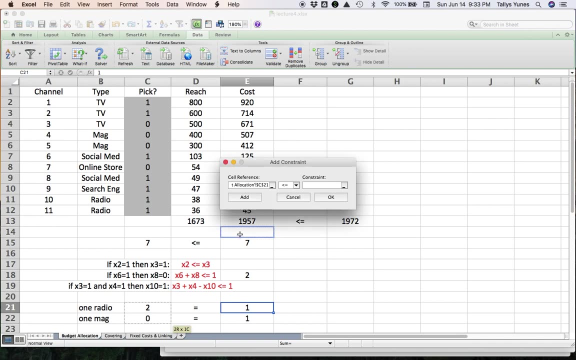 you wanted one yes and you have no yeses for magazines. now let's implement these constraints in solver and solve again. just to see what happens. out of curiosity, let me add them here and I'm going to say I want these two things to equal these two things here. 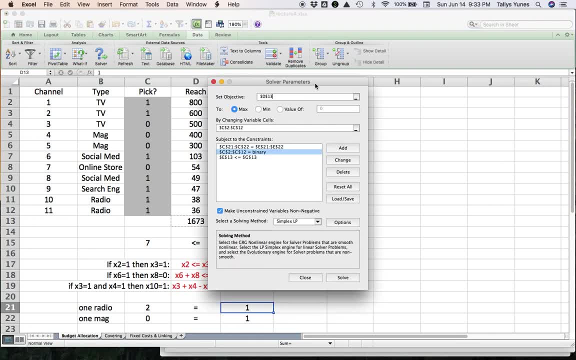 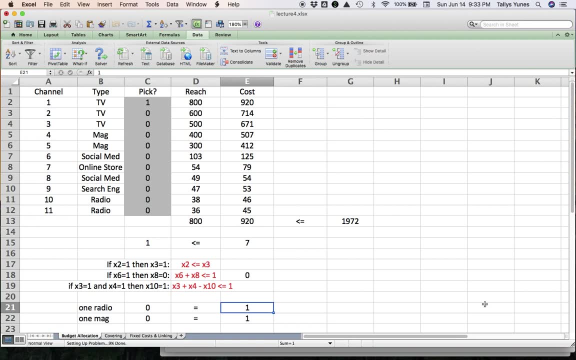 and if we solve that, let's take a look and see what happens. and again, this is going back to that thing that I mentioned: all the time, as you solve these optimization models, you never solve them only once, because you run them once and you look at an answer. 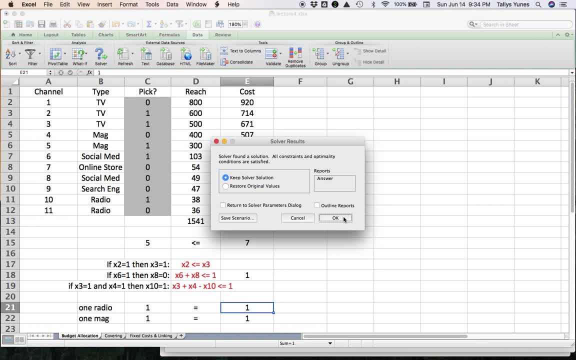 and you start to have other questions and you learn something about your problem. you realize you know what, now that I see this, I really want to have one radio and one magazine right. and then you add some extra detail, solve again, gain more insights and keep going, and this is the nice thing about. 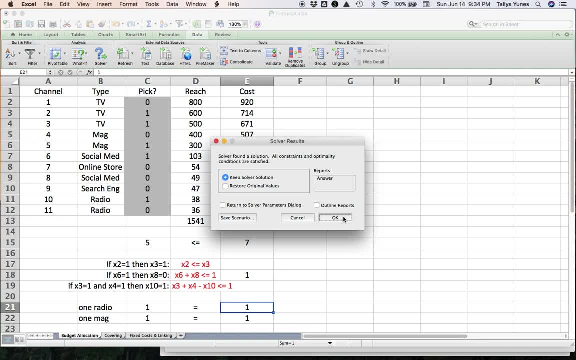 having these models, because you can play with them, change the data, learn about your problem and eventually, you know, converge to a solution that really satisfies your needs. so let's see what happens here. we, as we wanted, we obeyed, right the conditions we impose. there's exactly one radio. 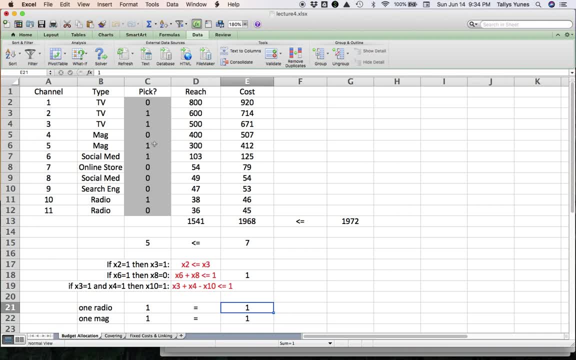 and one magazine, and the solver picked them in such a way that we would still remain within the budget, which we did, and we maximize the reach now. we are now reaching a million five hundred and forty one thousand people, and these are the ads we should advertise on. 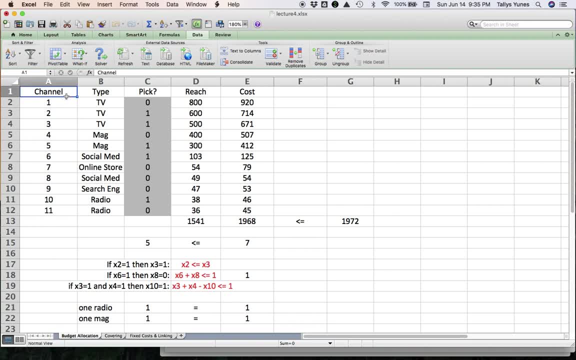 okay, so this pretty much covers the examples of logical conditions involving binary variables that I wanted to do with you. it's a very powerful elements to add to your optimization models: the idea of yes, no decisions. they're extremely pervasive in real life applications and, with the addition of logical 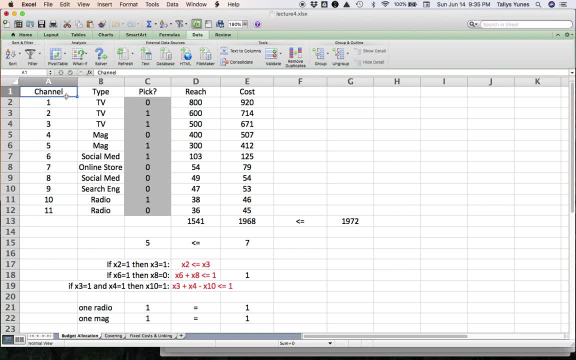 conditions. it takes your models to the next level. before we finish, I wanted to make one final comment that it something that comes up whenever I teach this, which is well, this is an if, then conditional. why can't I just use the excel? if function right, if I could do that, if. 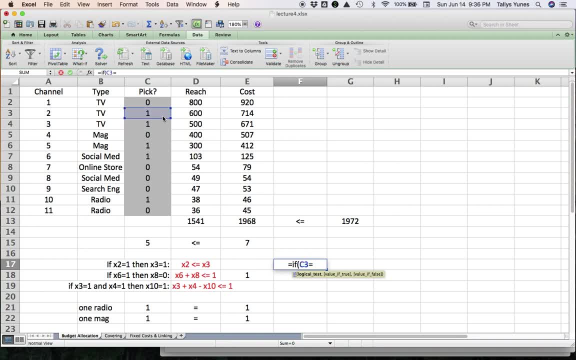 this variable equal one, right then. this variable equal one. that's an. if, then in excel, why do I have to implement it like this as opposed to like this? well, the reason is the following: this formula here is a linear formula, right it? if you were to plot the set. 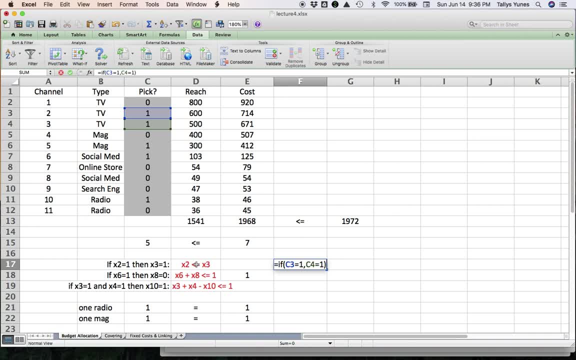 of solutions that satisfies that formula. they are on a plane. if you add this formula to your excel model, it transforms your model into a non-linear model, because an if function is not a linear function. what is a consequence of that, or the consequence of that, is the following: 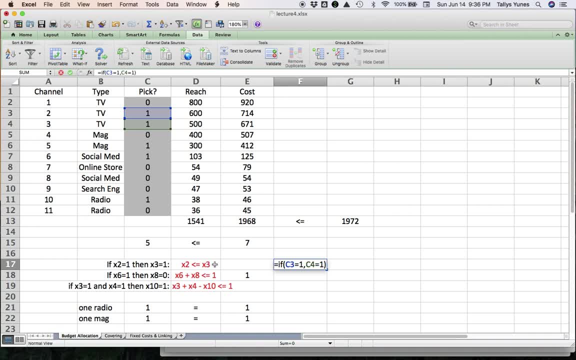 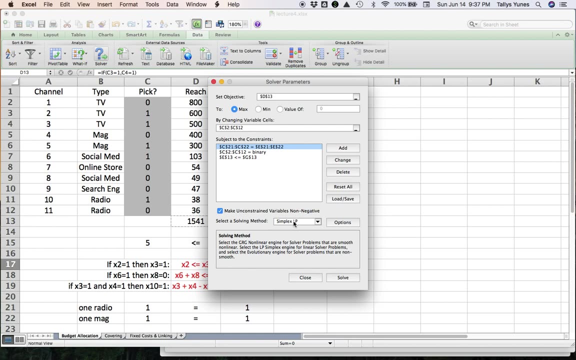 excel solver. if you have all your constraints linear, it allows you to use. it allows you to use the solver that we've been using, called the simplex lp. this solver guarantees that it will find for you the optimal solution if you have to change your model to include non-linear. 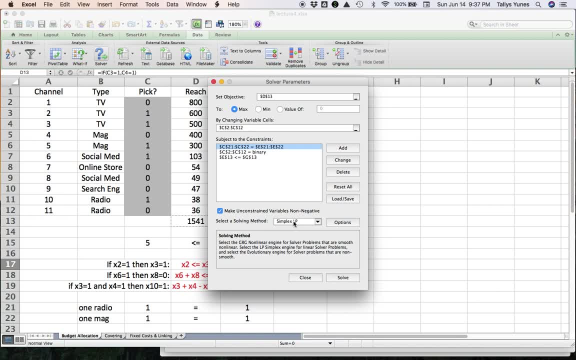 functions such as the if function, the max function or some other more complicated calculations such as square roots and logarithms and things like that. you then have to switch from the linear solver to the non-linear solver, and the non-linear solver in excel does not guarantee anymore.